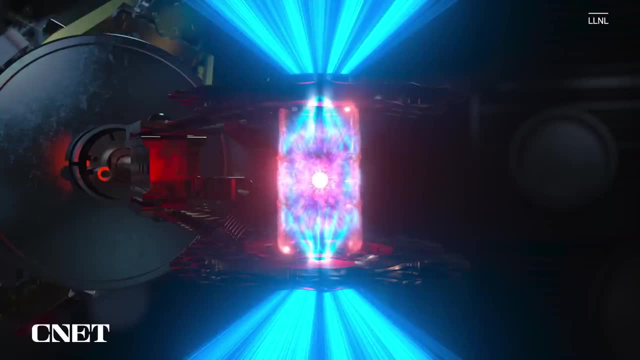 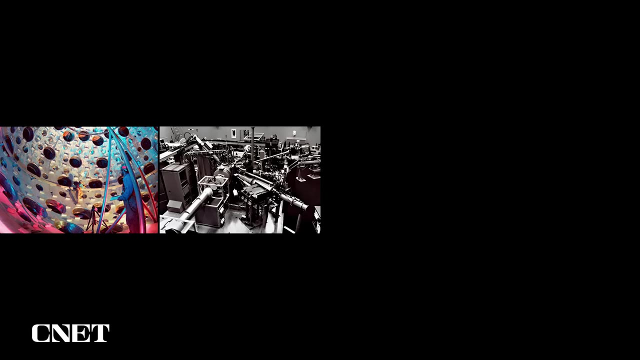 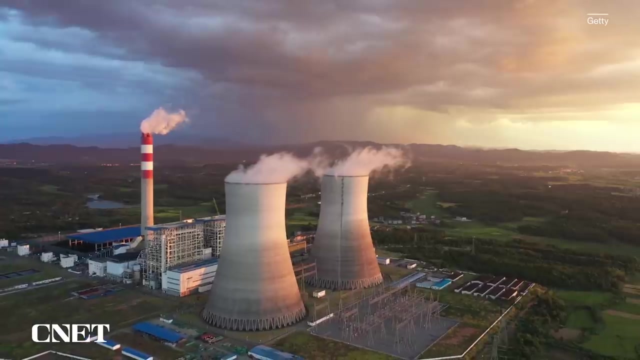 the amount of energy created when those lasers hit the target than it took to trigger the reaction. That's the first time that's ever happened. Scientists have been chasing sustainable fusion for decades. because of what it promises: There's no release of carbon, so it could drastically change the course of human-caused climate. 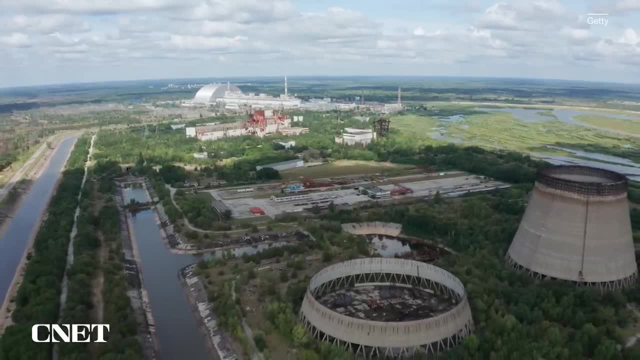 change. It's safe- there's no risk of a meltdown that comes with our current nuclear fission plants. And it's virtually limitless because it only relates to the amount of energy that's produced by the laser. And it's safe- there's no risk of a meltdown that comes with our current nuclear fission. plants, And it's virtually limitless because it only relates to the amount of energy that's produced by the laser. And it's virtually limitless because it only relates to the amount of energy that's produced by the laser. And it's virtually limitless because it only 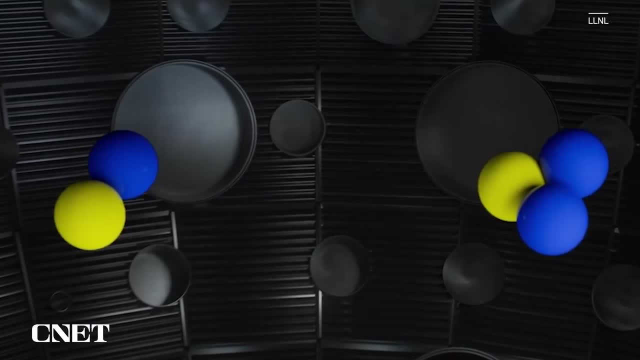 relates to the amount of energy that's produced by the laser. So in this case, fusion requires hydrogen, the most abundant element in the universe, And fusion requires hydrogen, the most abundant element in the universe. Fusion occurs when two lighter elements like hydrogen merge into a single heavier element. 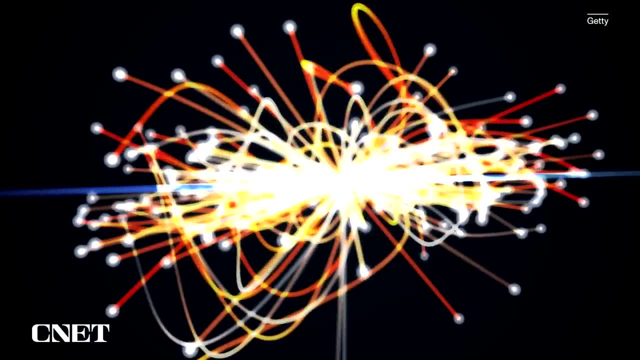 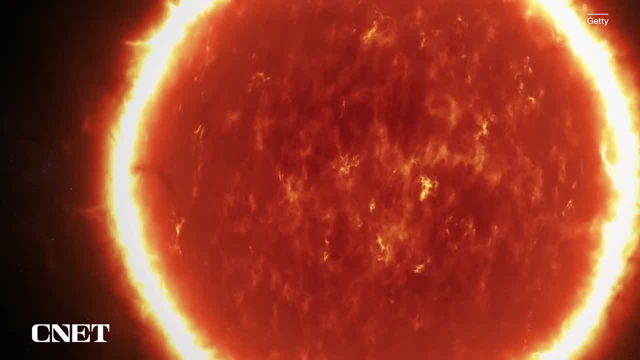 In this case, those hydrogen atoms merge to create helium. The process of the atoms fusing together is nuclear fusion, the same kind of reaction that causes the sun to release energy. What we do here is called inertial, confined fusion, where we take a small amount of fusion. 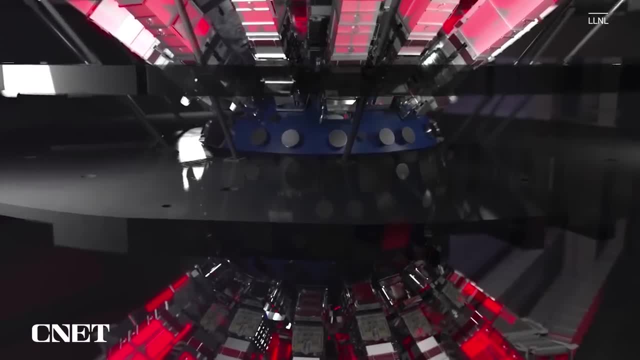 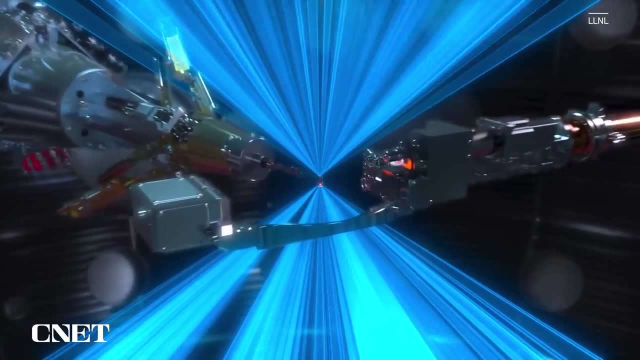 fuel and we take lasers, In this case 190 liters, 192 beams that all add up to about 2 million joules of laser energy. deliver that over billionths of a second and have that laser then enable that pellet, that fusion pellet. 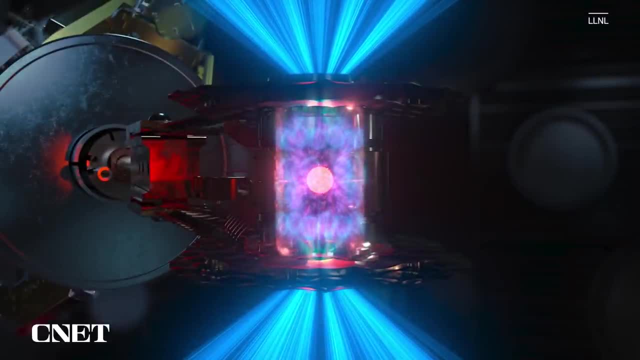 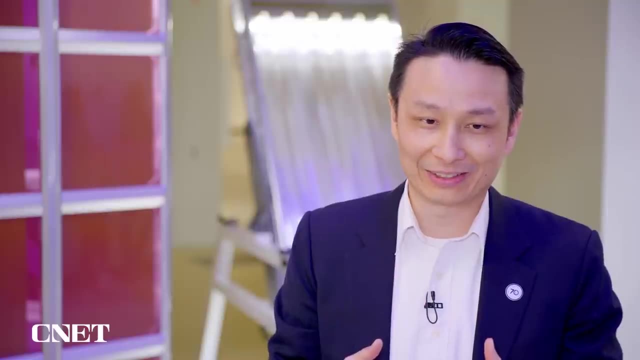 to go from millimeter scale to down to 100 micron scale, so width of a human hair type scales- And if we can do that and if we do it right, we then get to these conditions that are more than 100 million degrees hotter than the center of sun pressures, that are in the billions. 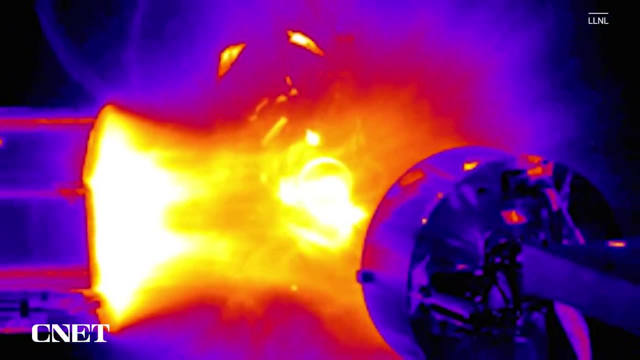 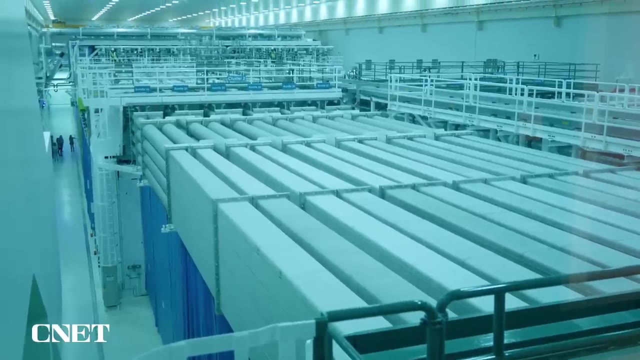 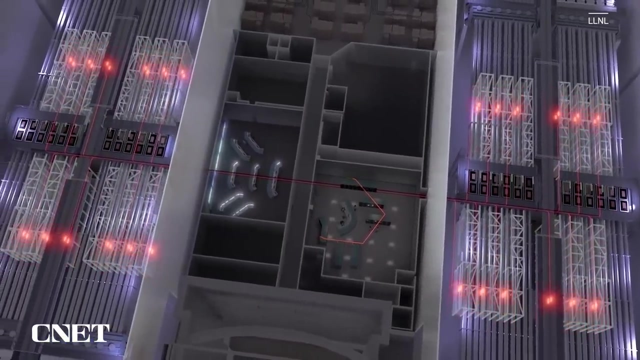 of atmospheres, And if we do all this right, then we can start what we call fusion ignition. This is where it starts. You're looking at one of the facility's two football field-sized laser bays each containing 96 individual beam lines. The beams start with just a small amount of energy. 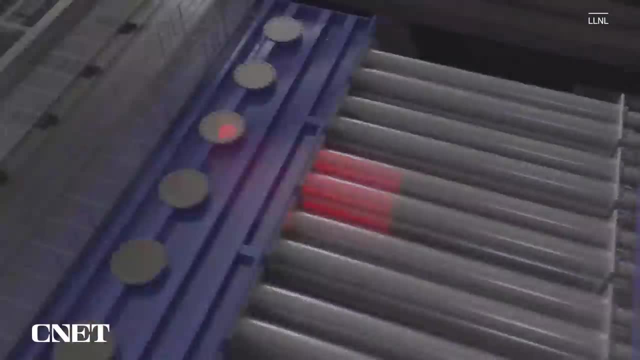 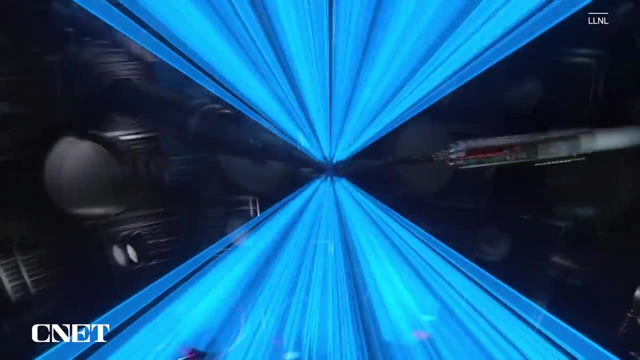 This is where they come to get amplified a quadrillion times. Now it's time to head for the target chamber, and scientists hope that energy will trigger a fusion reaction. So this is a one-tenth scale model of the target chamber inside that we're about to see. 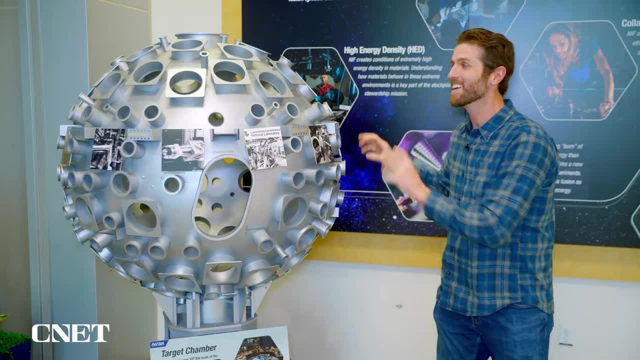 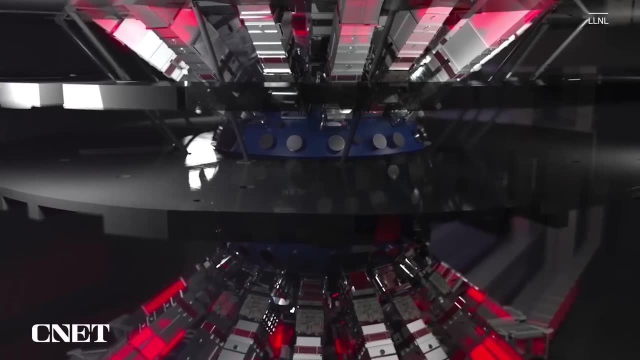 A scale model, Andy, would be about four inches next to this thing. Now you can see these ports along the top here and along the bottom here. Those are the quad ports. Those are for where the lasers, those 192 lasers- actually come into the target chamber. 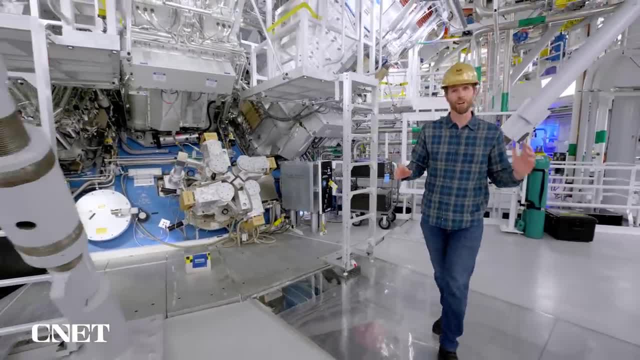 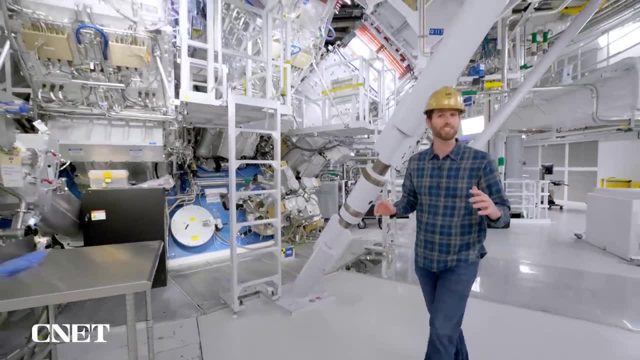 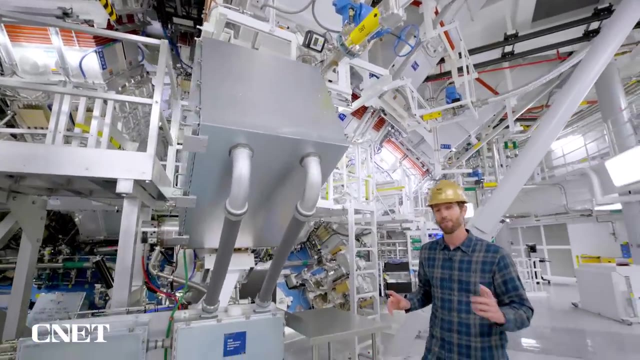 And this is the real thing. This is nearly 300,000 pounds of aluminum. This is where it all happens. Above me, you can see these quads. Those are groups of four out of those 192 lasers that make up this entire facility In front of me. here, this is called Dante. They call it Dante. 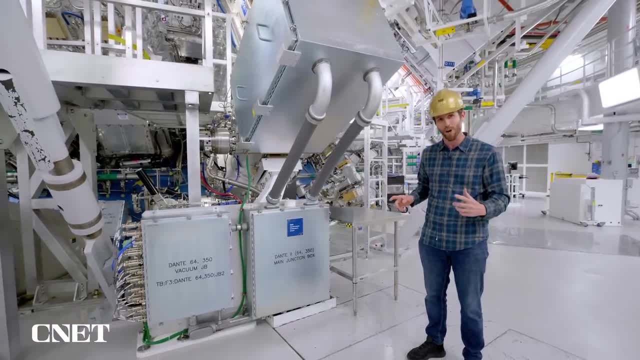 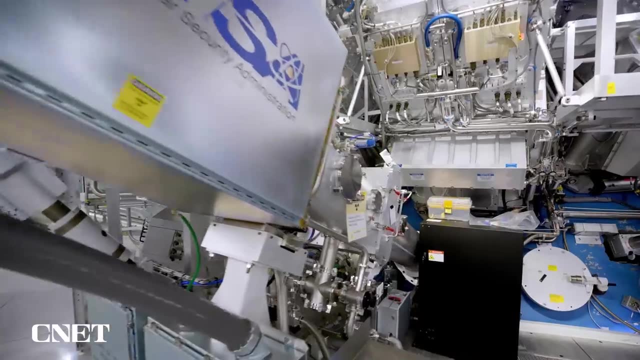 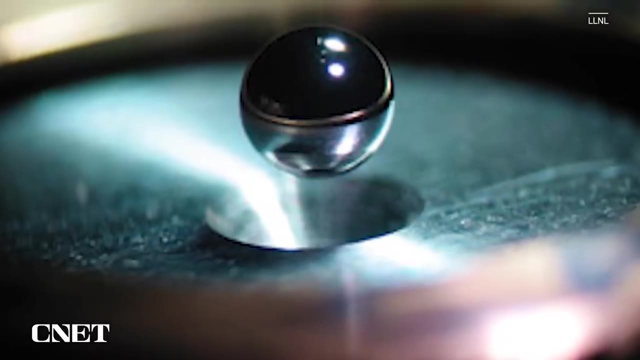 because it basically measures the temperature of that inferno that goes on when there's a reaction. Just how hot does it get? Every time scientists fire this up, this target chamber becomes the hot, hottest place in the solar system. And what does it do to a target about the size of a BB? 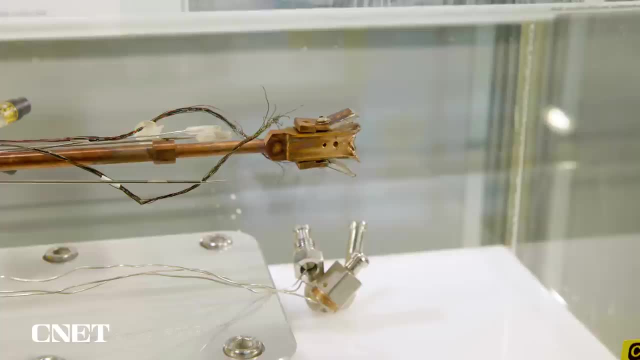 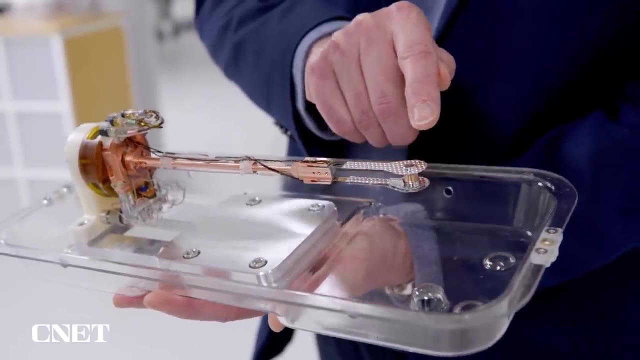 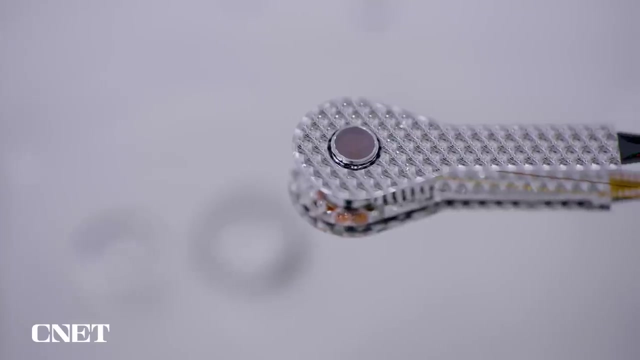 This is what's left of a target. from a previous shot I asked Gordon to show us what happens inside a target during an event. The laser beams are delivered to the target, which is inside this little few-millimeter hole inside the gold can. Half of the beams- 96 beams- are delivered in the top. 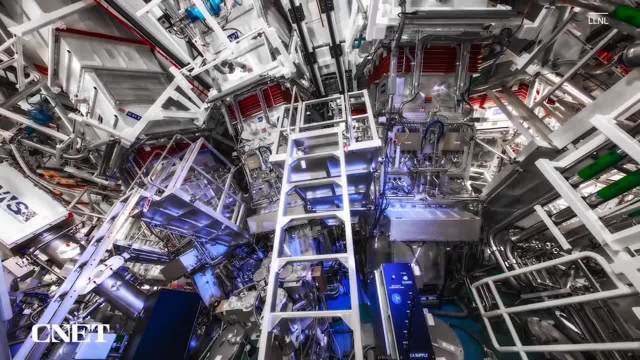 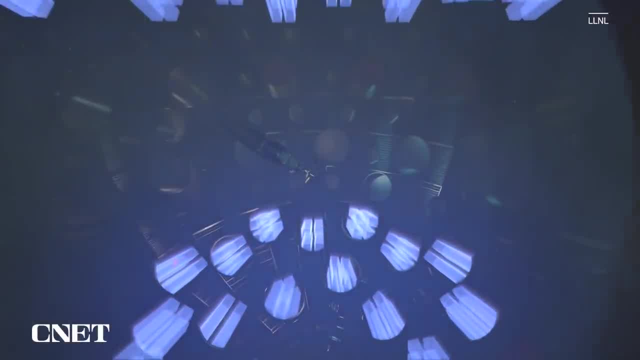 Half of the beams are delivered in the bottom. December's event required a lot of work to get the laser beams delivered to the target. A little over two megajoules of energy to trigger the reaction, producing a little more than three megajoules. That's about a 50% gain. 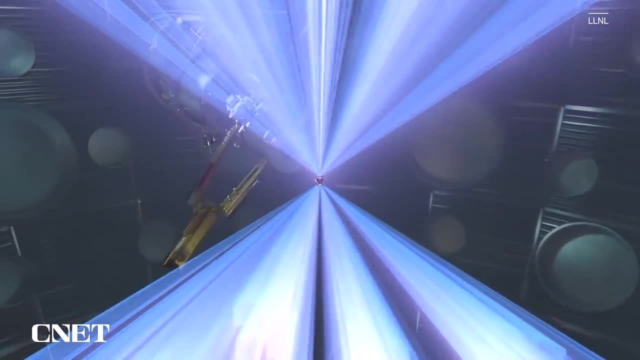 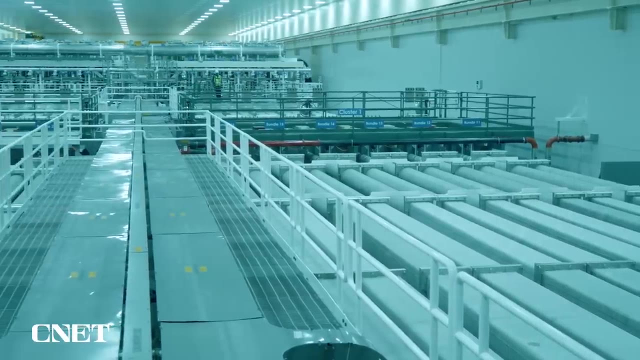 and that's why scientists are excited. But those numbers aren't the whole story. It took about 400 megajoules to operate the lasers that would ultimately hit the target with those two megajoules of energy. But scientists point out NIF was never designed. 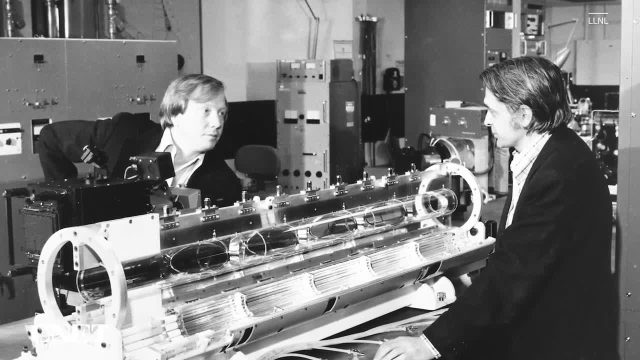 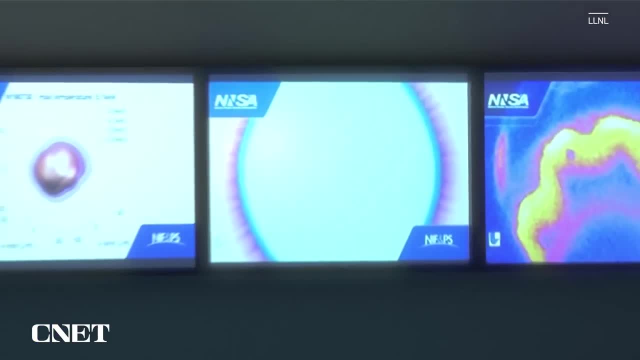 to be efficient, let alone a power plant. It's a scientific instrument designed to prove what's possible. In fact, NIF's research isn't intended for energy production. It's to provide data ensuring that the United States' arsenal of nuclear weapons is safe.